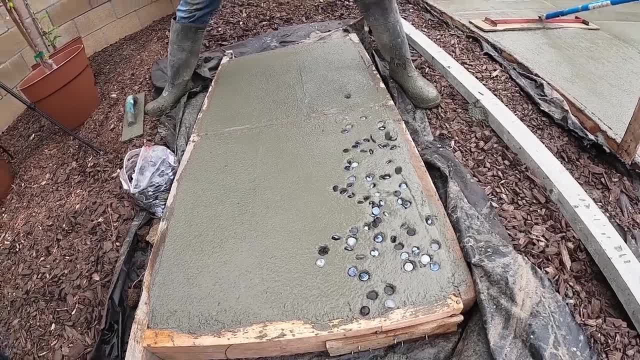 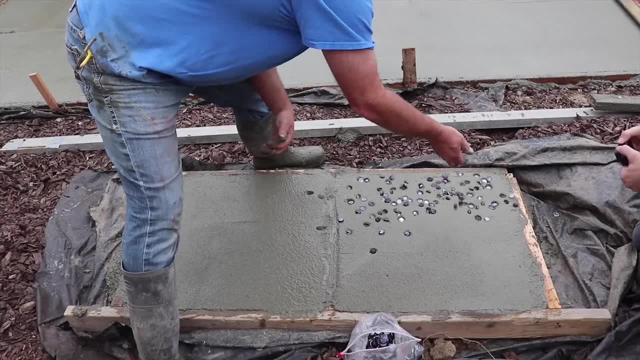 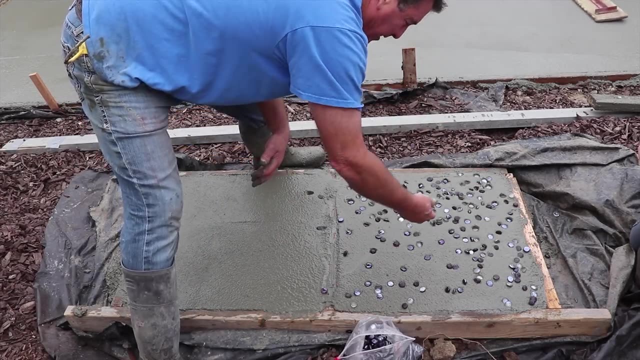 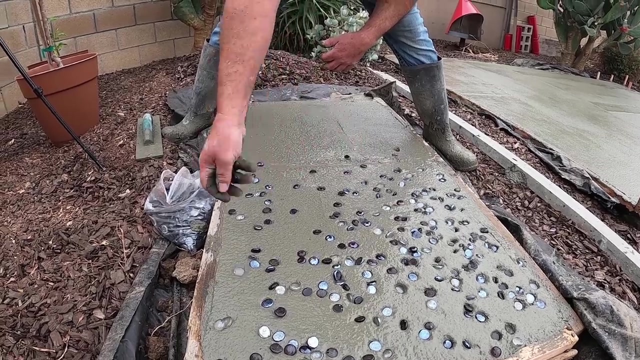 see how they're sinking way down just by dropping them. We'll just do this one. We'll do this one early and we'll wait on the next one and go a little bit later, because I'm going to lose a lot of glass. This is pretty wet right now, So a lot of it's dropping down deep, never to be seen in. 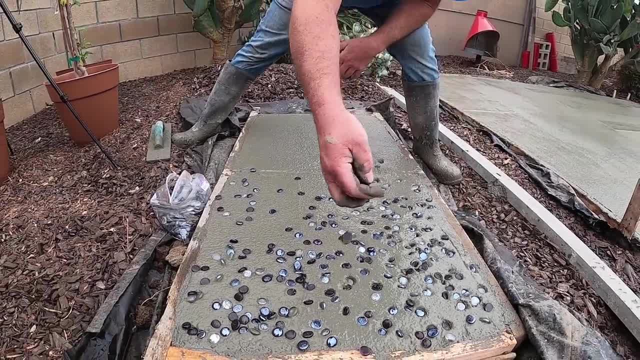 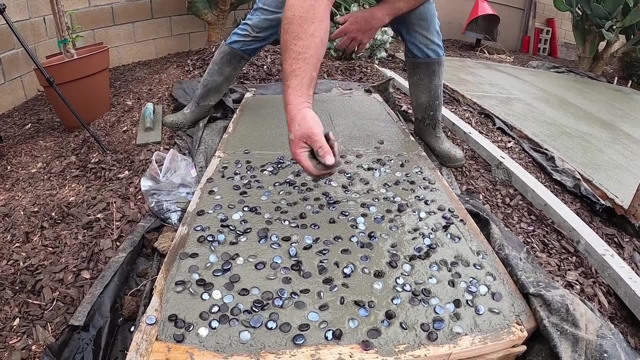 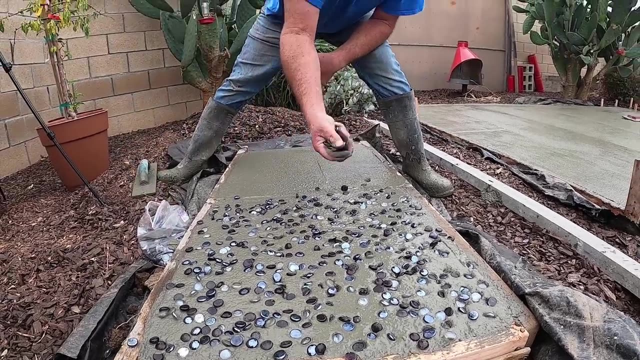 the sun again. I just want the stuff on the top really Look at this process that we're doing. It's going to take at least four hours minimal in 70 degree weather, no sun about you know. four hours, four to six. 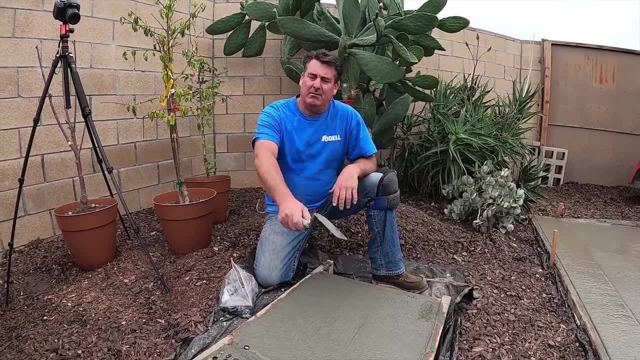 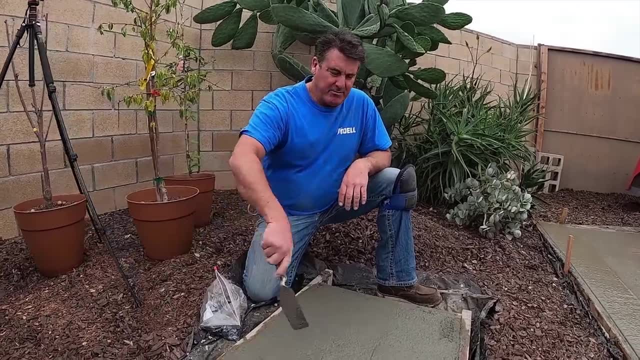 This is an hour later after the initial lay down. We've already put a glass coating on the first stepping stone And this one here we're going to go with just like a lazy river pattern going through it of the glass. So I'm 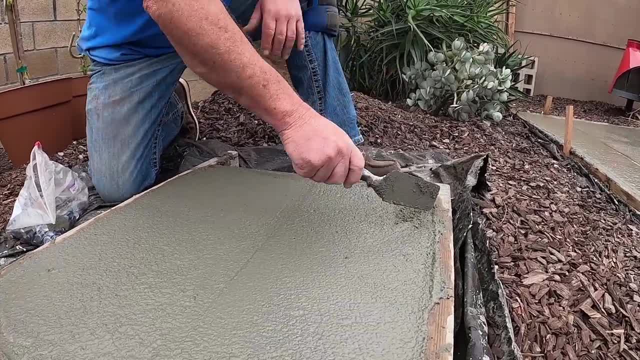 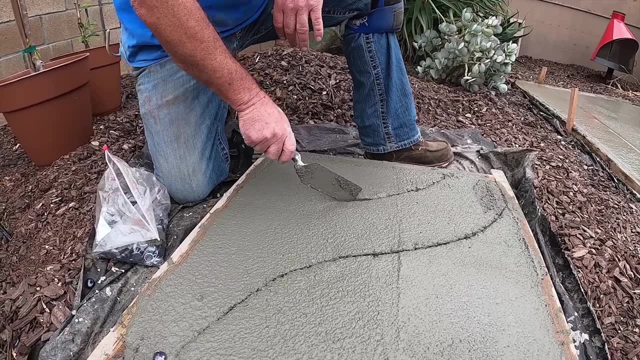 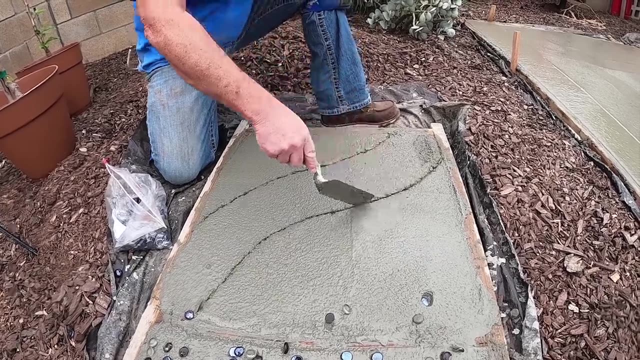 going to draw it out first, the pattern we're going to try to get. Just start here. We'll just do a lazy S Start right here. Just try to maintain that. There we go, See how we have that little shape there And that's going to be the glass area. 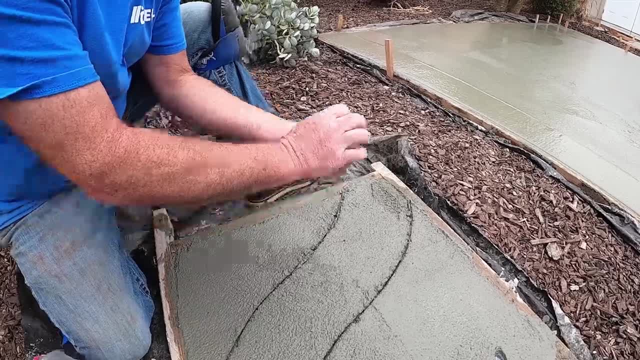 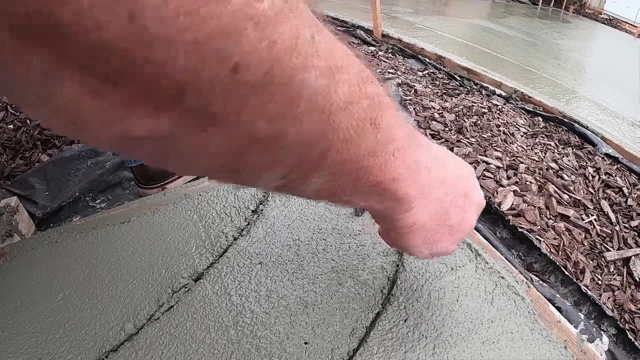 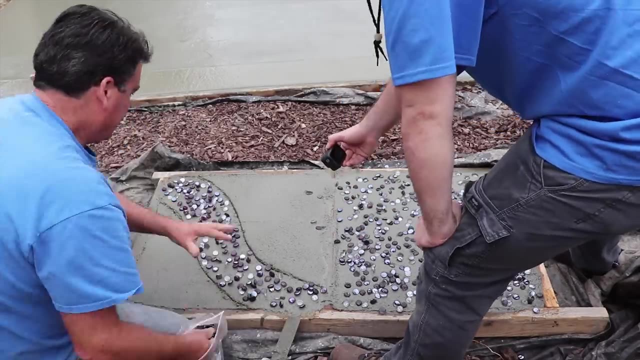 Now the tricky part: getting the glass where I want it. Have to take my time on this. Get it just right. Whoops, see that Almost messed up. This is going to go back in there and we're going to draw the glass. But I don't want to mess up the tip of the glass. So I'm going to start with that second taking piece and then we're going to go back in there, and then we're going to come back in there and we're going to draw the second piece. So look at this one here. This is what we're taking on. If you're gonna draw on this one, you can just go ahead and pull it up a little bit. The other side up here, You're going to drill it out like this to make it, just so that it doesn't fall in the bottom. 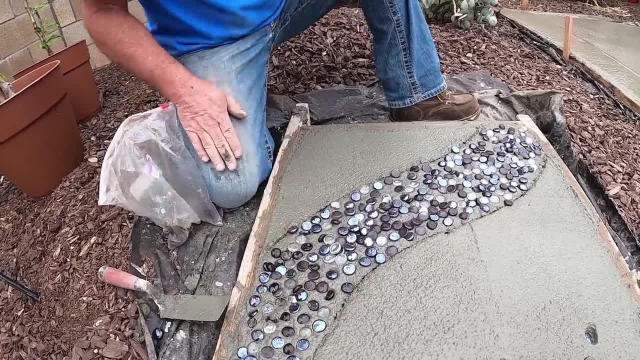 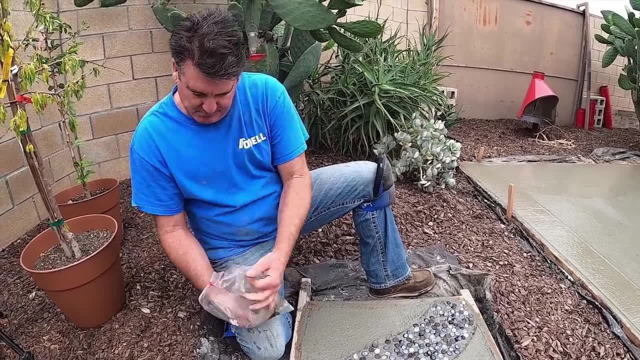 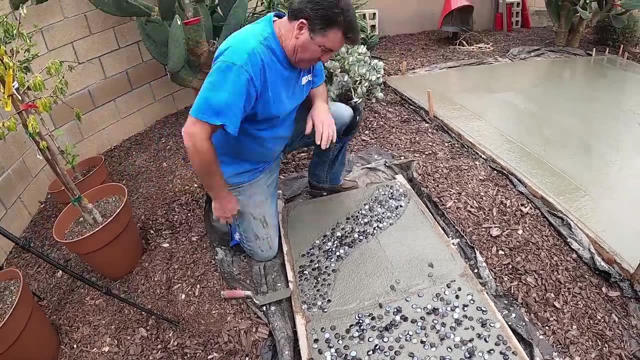 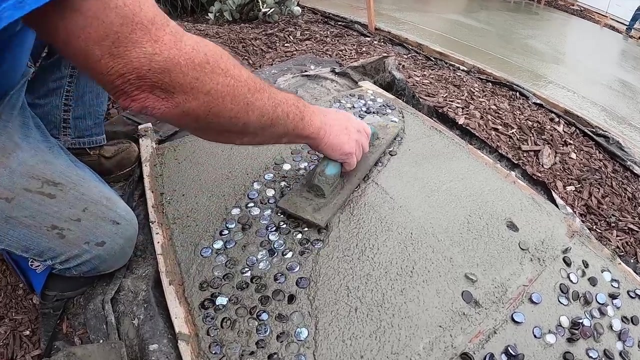 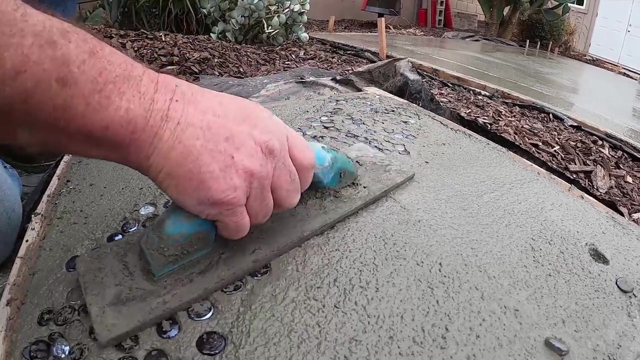 This is kind of setting them so they don't move around on me. All the glass is gone, tap it in. We'll try to get this all the way flush. You don't want these to fall out later. We're going to actually bury them, And then what we'll do later. 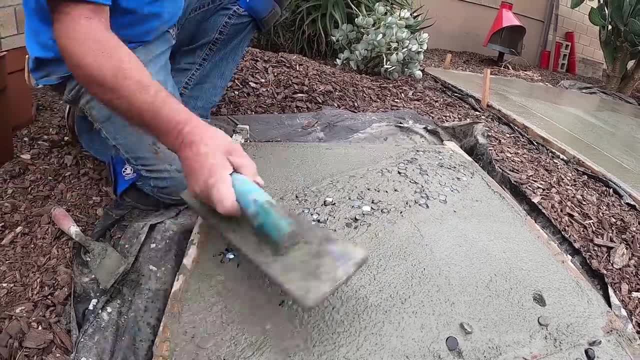 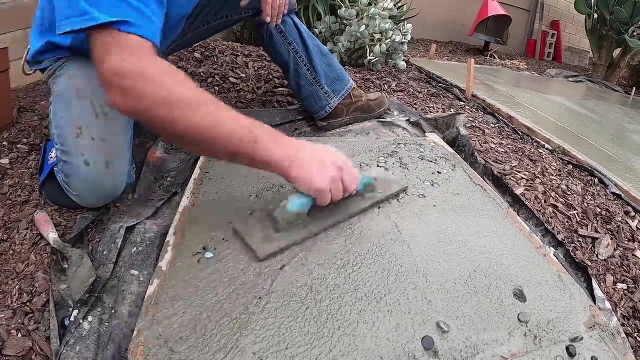 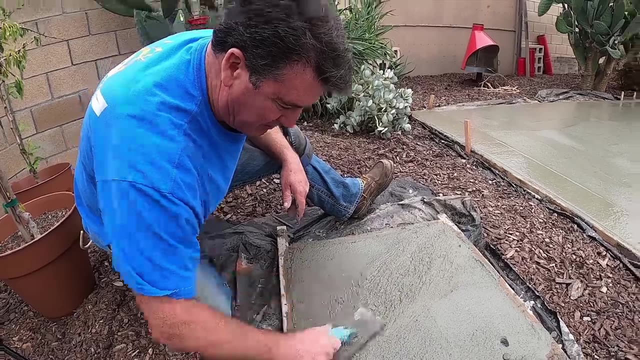 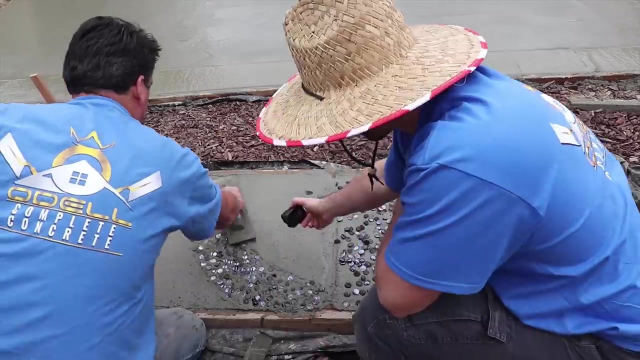 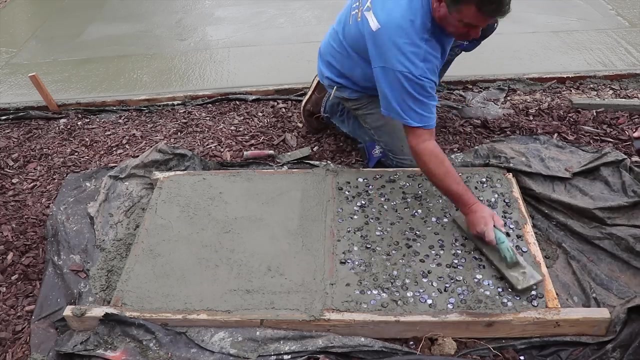 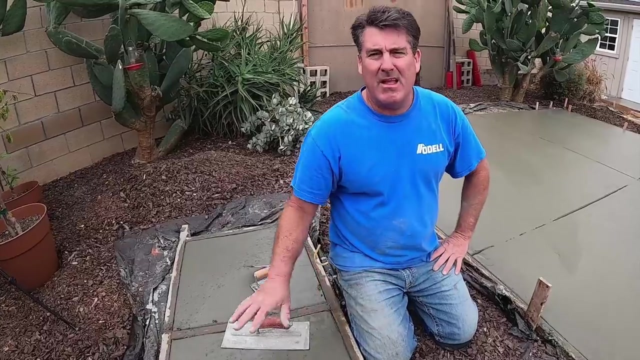 We'll expose them by rinsing with water. We'll do that probably about three hours. Right now, all the creams going over these glass beads. The glass has disappeared. The interesting part is the sink. We'll see when it comes back when we do the rinse. All right, we're back on it, and now it's three hours later. 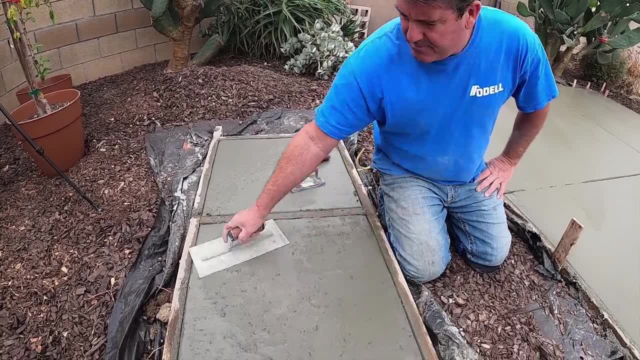 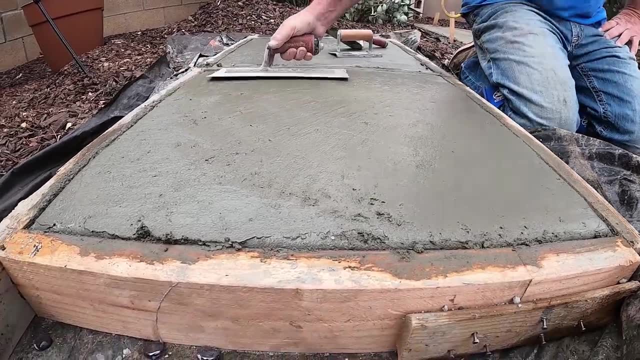 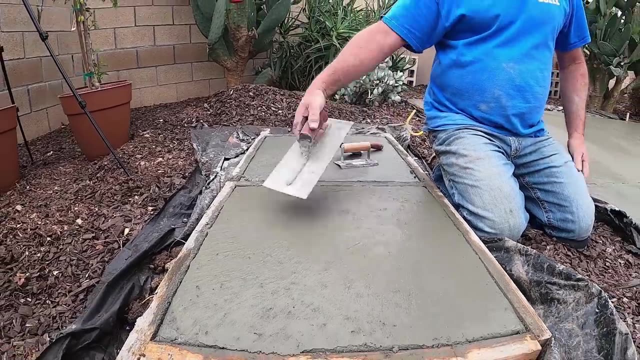 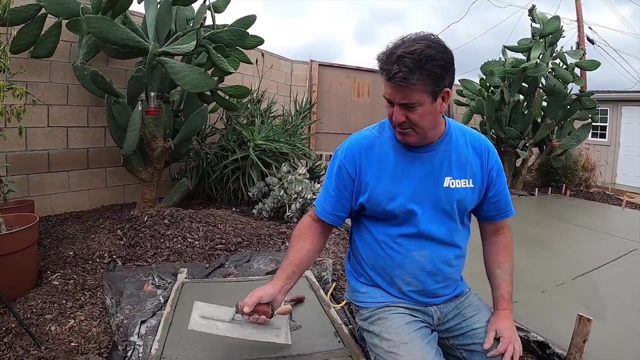 And we'll be troweling it one more time and edging it And then we'll see what happens. So you notice that the glass beads aren't popping. The cream's not really popping off of them As much as they were earlier, because it's a little drier now. 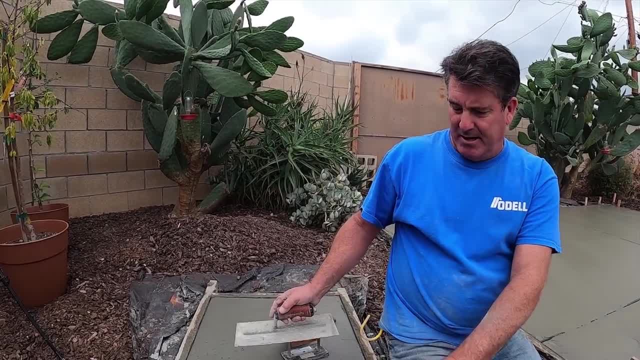 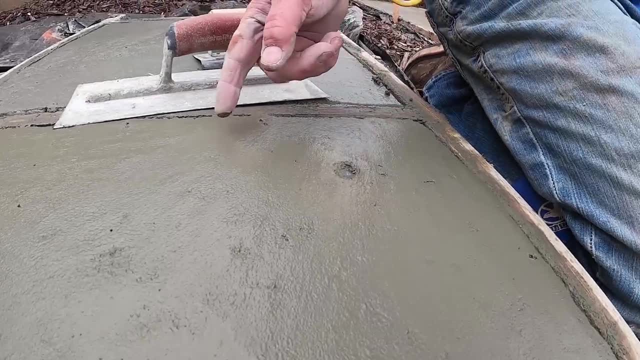 Once we can get a perfectly smooth finish And you can't see those beads starting to pop. See the little rock pockets on top of, Like if we were to clean this off. see there's the glass. so what's happening? because it's still a little wet to get your final trowel. 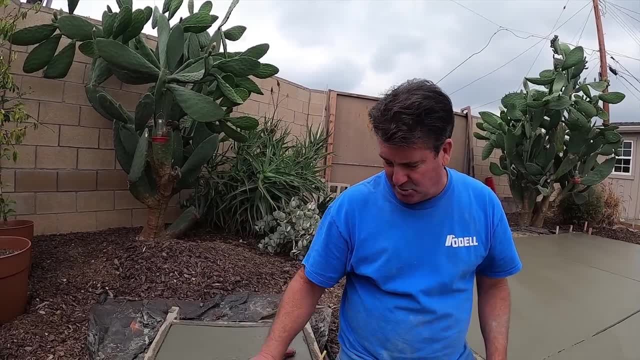 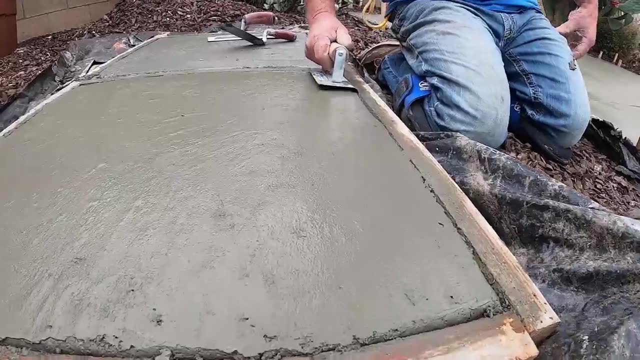 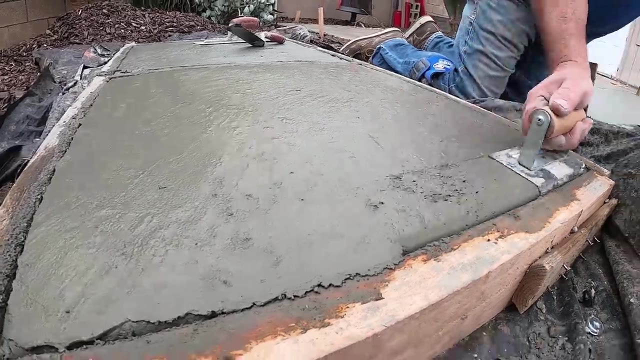 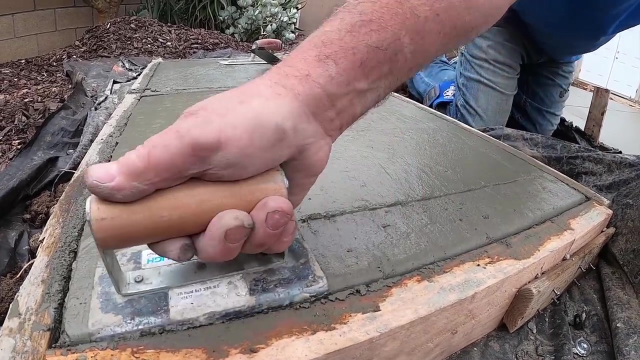 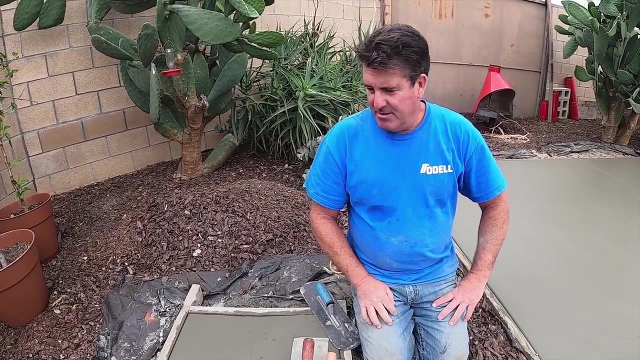 is the rocks. the cream is just kind of rolling off the top when you pass a trowel over it. so basically it's just too wet. so all right, we're back on it again four hours later. this should be my final pass, so just edge it, trial it one more time, then i'm gonna let it set another hour, so we'll be. 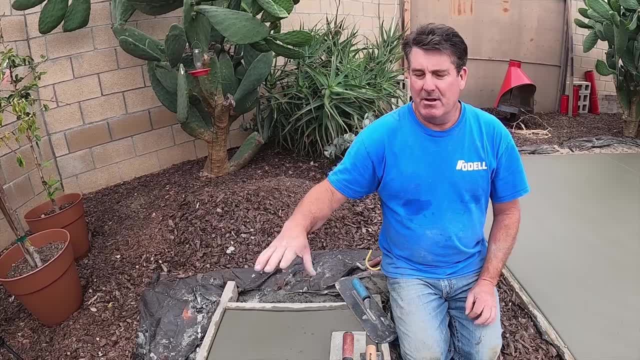 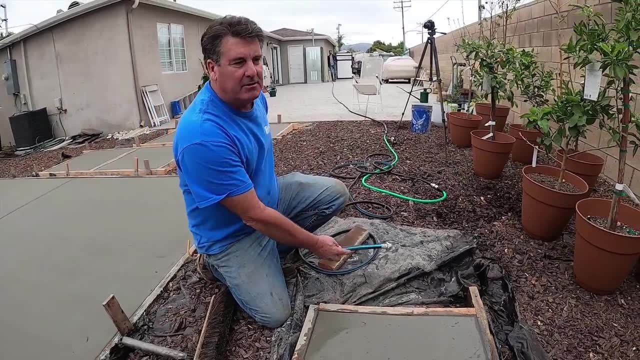 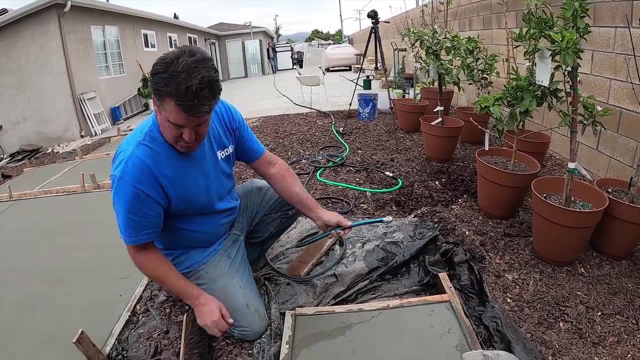 a good five hours total into this, but once i do the rinse i'll give you another timeline on that. here we go, all right, how many hours we into it now let's take a look here: four, four and a half hours. let's see if it's ready. i'll just put a little water on it. 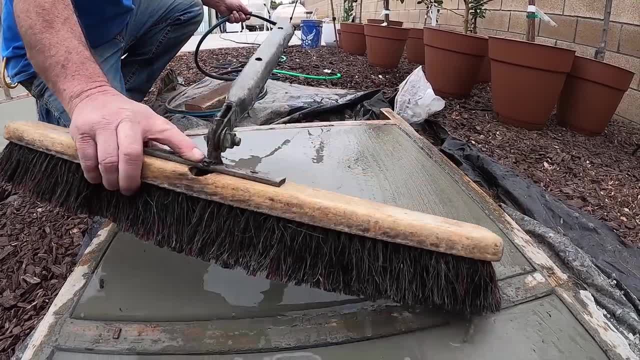 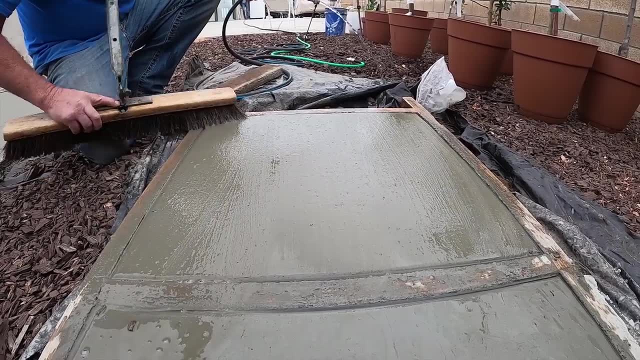 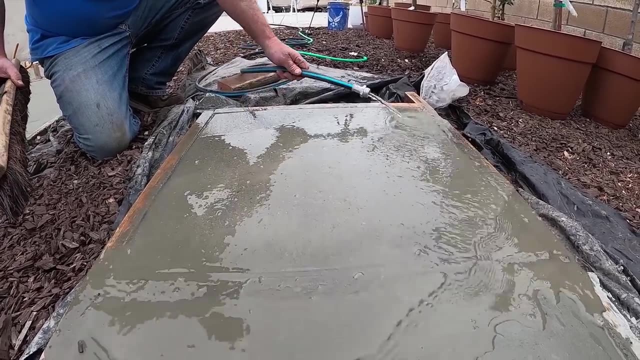 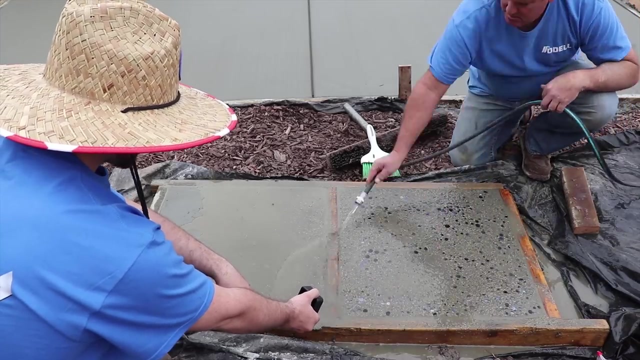 start with, loosen it up. loosen it up with this horse hair broom. get it loosened up. do another light rinse. see where we're at. oh, look at that fiber mesh coming up. all right, that was pretty interesting how that fiber fiber mesh just rolled off the top. 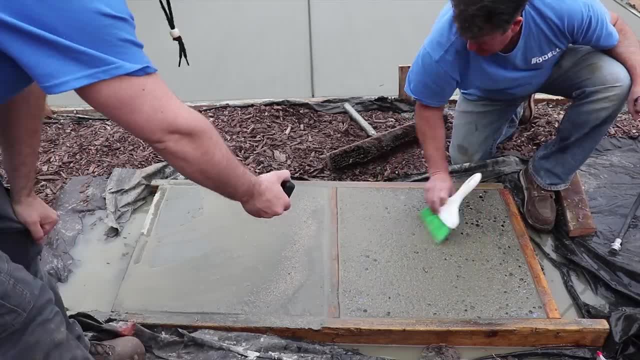 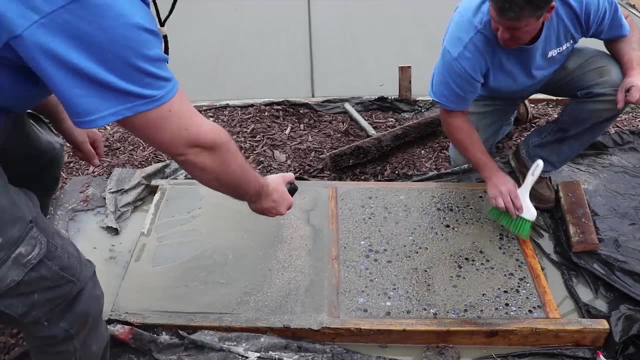 that's when you know it's actually in there, when you can see it. so i ended up going with a nylon brush, a little bit stiffer, because i kind of almost waited too long to rinse this. actually, i mean, i couldn't wait to get this out of the water, but i'm not even sure how long it took me to do it. 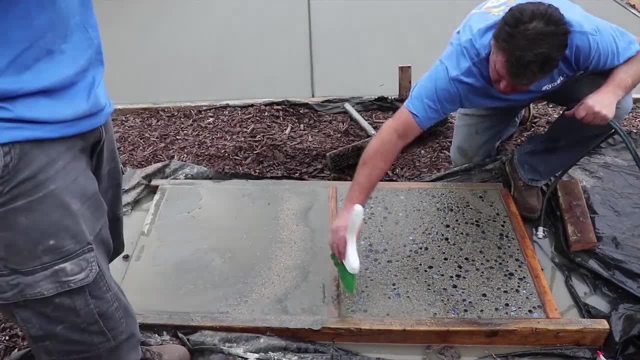 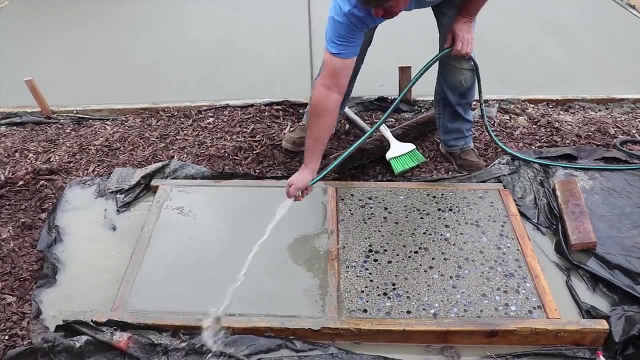 i think it's about 15 minutes. i think i probably went about another 15 minutes early. but it's better late, you know, than early, because if you go early all these beads will just fall out. you'll have a real mess. so i had to scrub a little bit harder because i went late. but 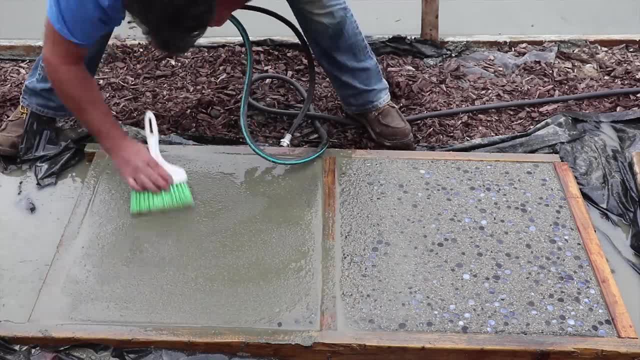 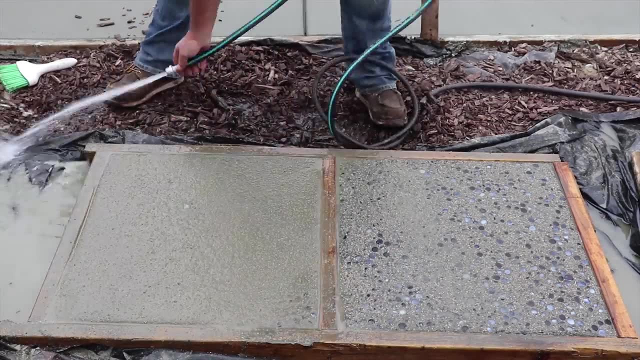 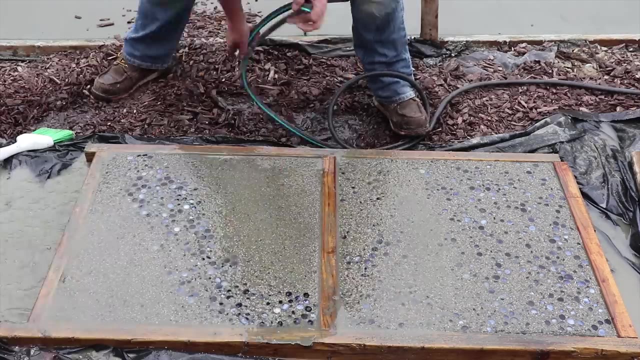 you know the beads are well embedded and they're not coming out. you know they're not coming out. strip the forms, separate them, give it a good cleaning and we'll seal them. The nice thing about these stepping stones: if you're considering doing something like. 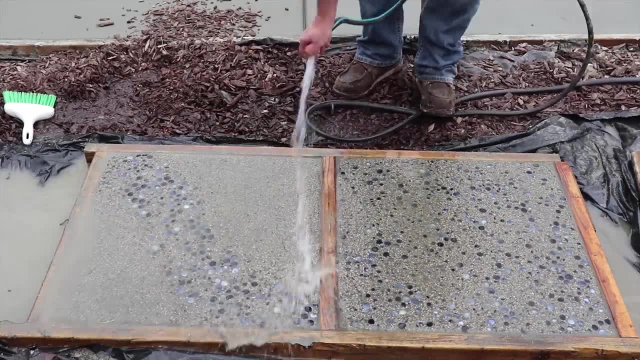 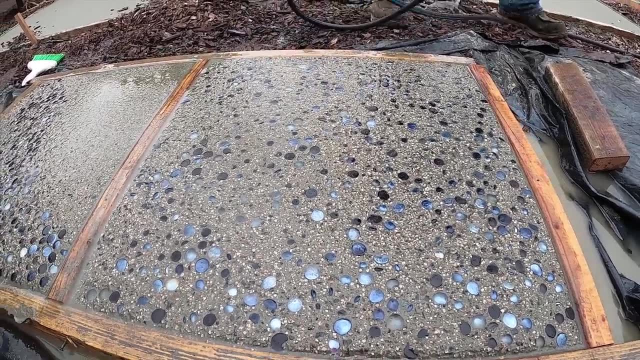 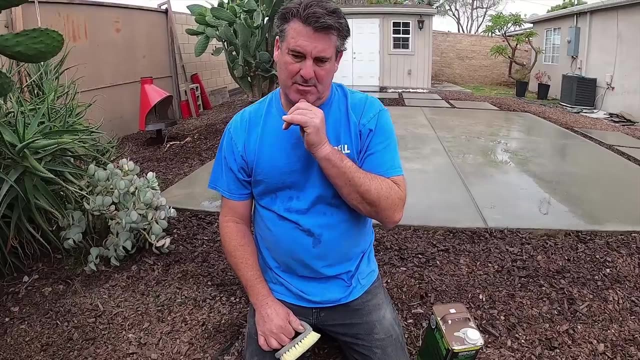 this on your own at home. you don't really need a concrete truck and a pump hose and all that. You can do it with some typical bag mix. you know quick crete, Any bag mix, concrete pre-mix will work just fine. 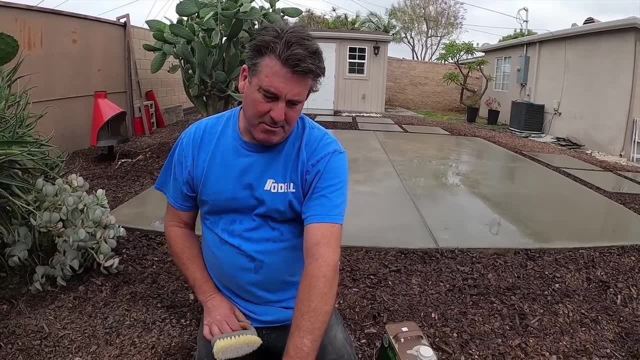 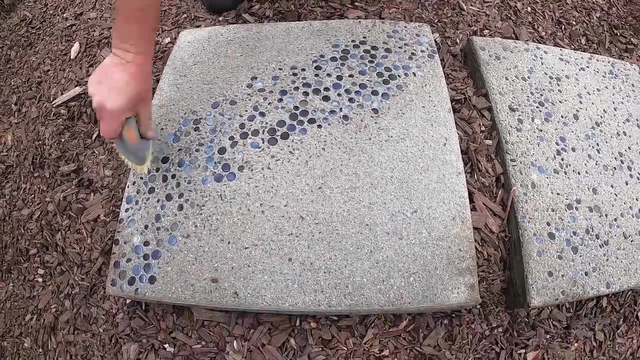 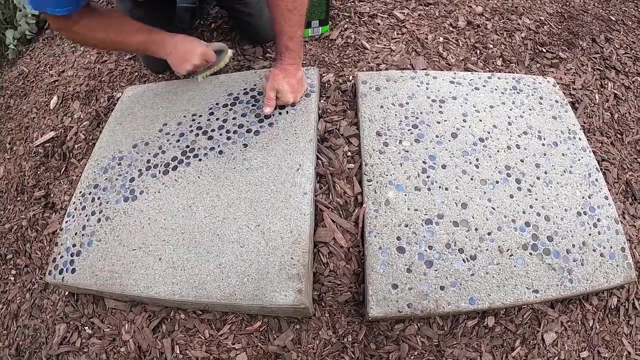 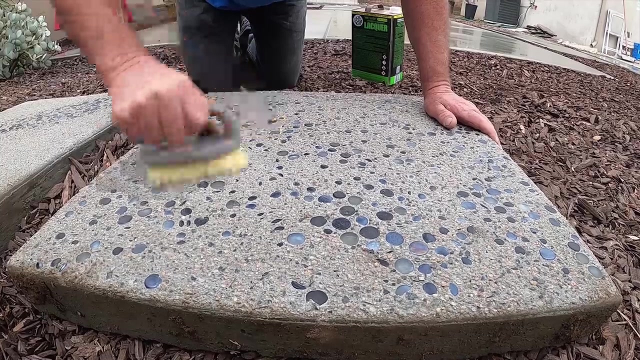 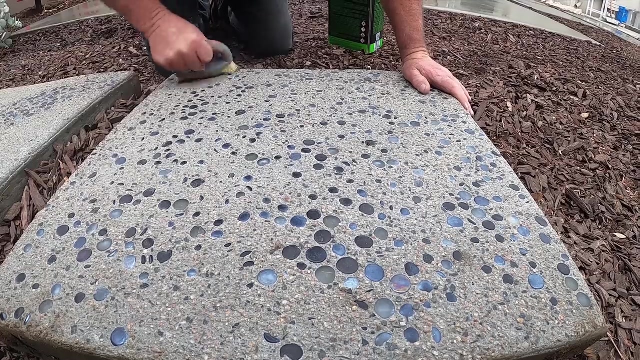 All right. second day We just stripped the forms on this. now I'm just going to brush it. get any residue off of it. It might still be on these glass beads. I'm just going to brush it. Okay, we did this pretty quick. 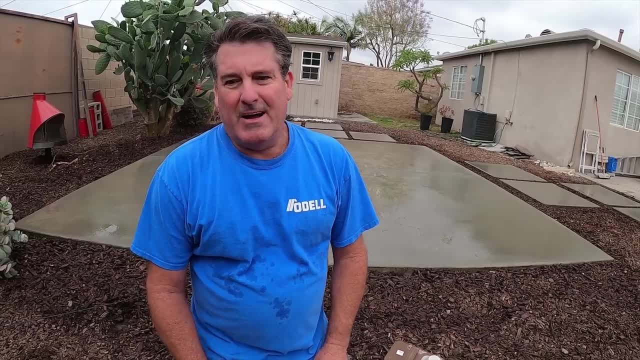 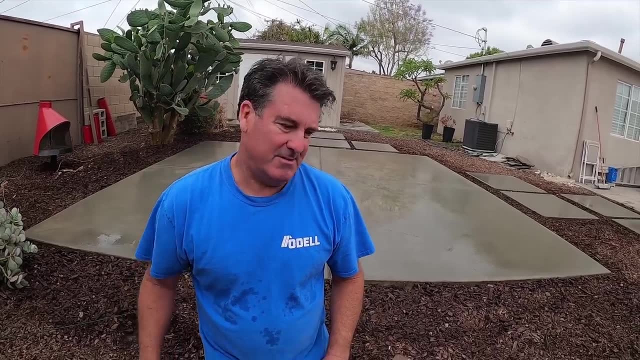 Second day: we're going with the sealer. We didn't do the muriatic acid wash, We didn't neutralize it, We skipped all that went straight to the brush. Now we're going to go right to the sealer. 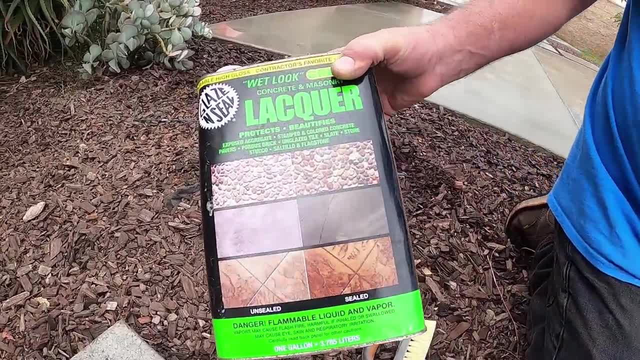 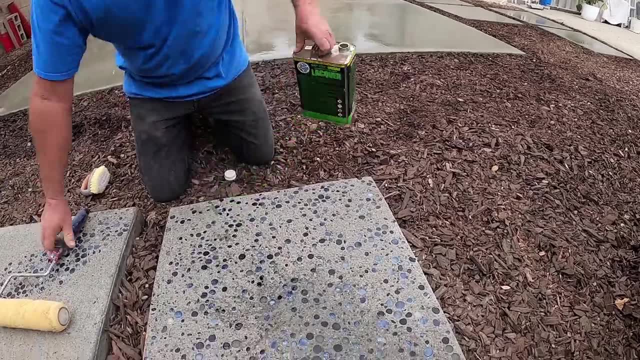 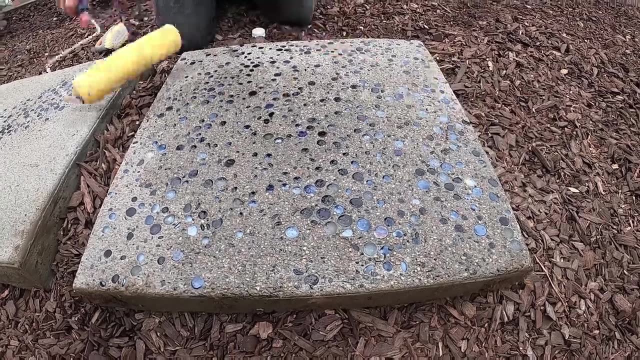 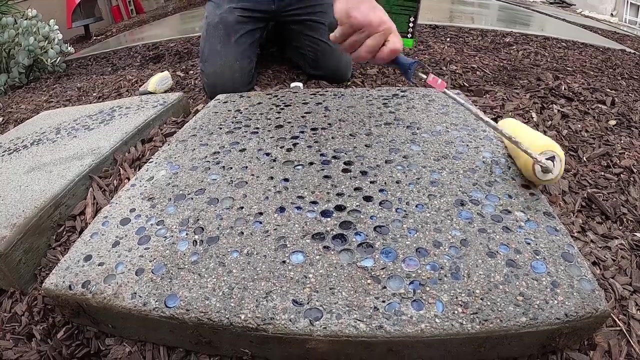 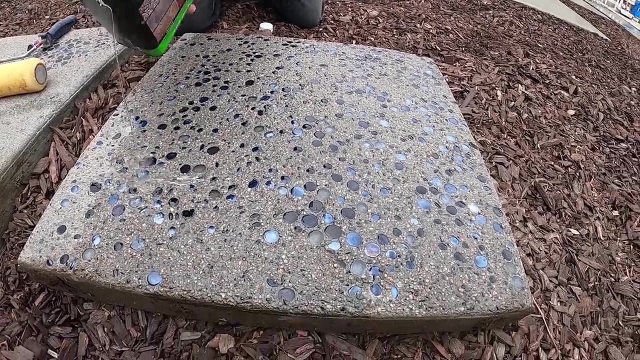 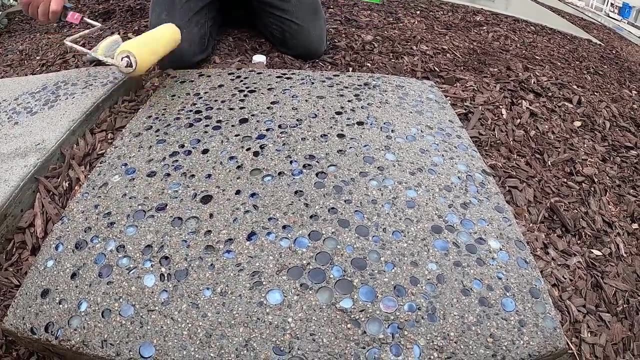 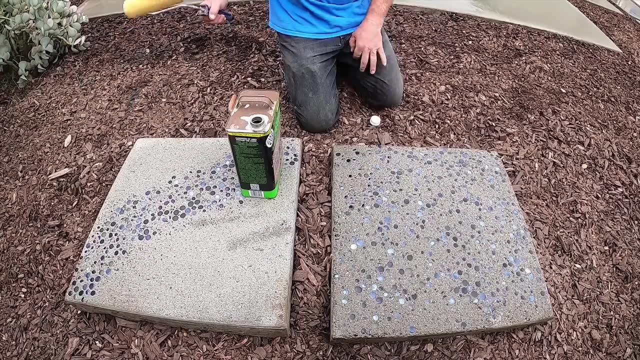 Available at Home Depot. Roll it around. Oh wow, That's a lot of sealer, That's a lot of sealer, That's a lot of sealer. Oh wow, this is really looking good. huh. Typically, you can't really seal this stuff the next day, especially a large area. 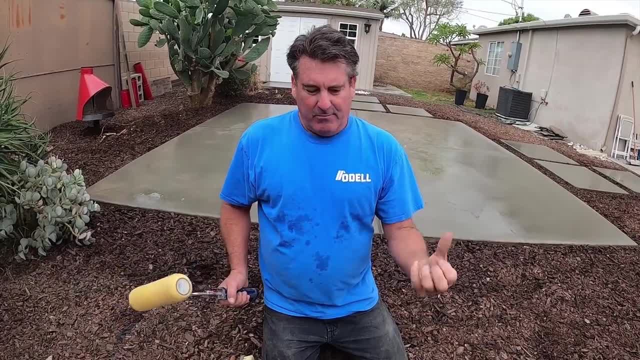 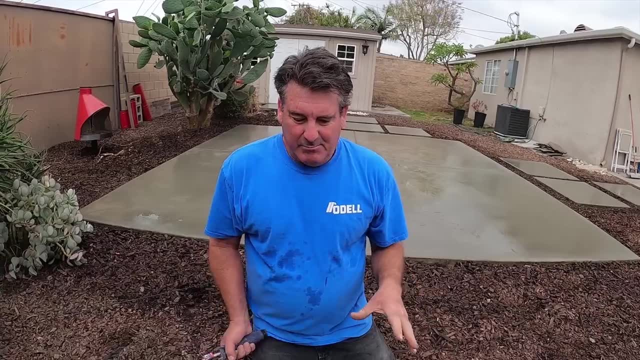 What happens is the water wants to evaporate out of the concrete. If you have water trapped in the concrete, it gets stuck between the sealer and the surface of the concrete and it turns milky white. But in this case that's the concrete area. 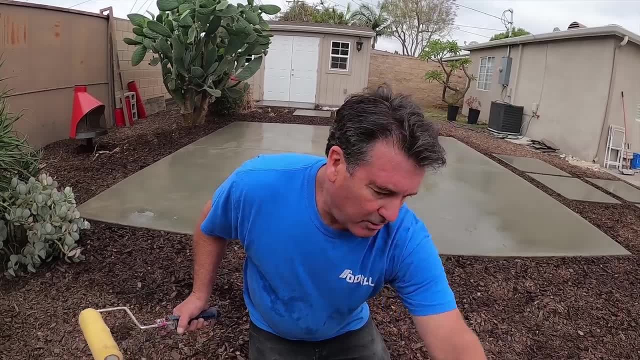 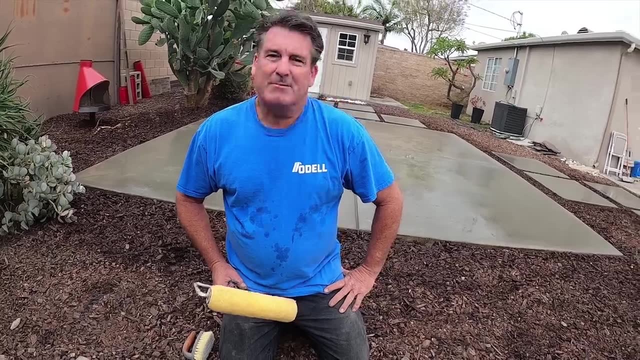 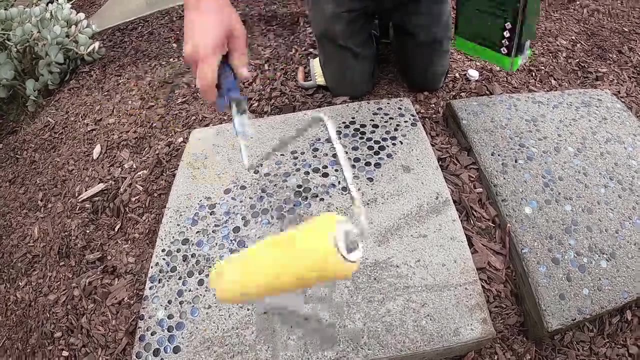 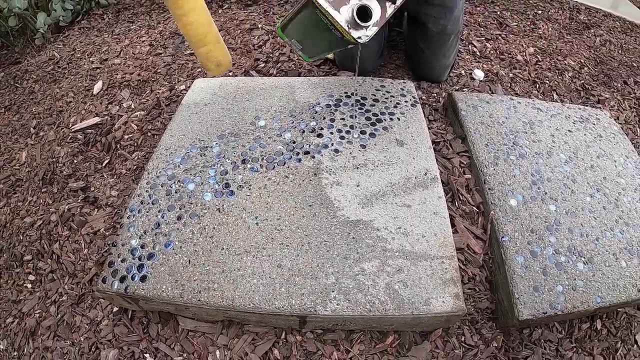 Because the concrete areas are so small and they can breathe all the way around it. we can displace any moisture out the sides. That's my hope anyway. We'll find out long-term, but I'm pretty sure we're good here.